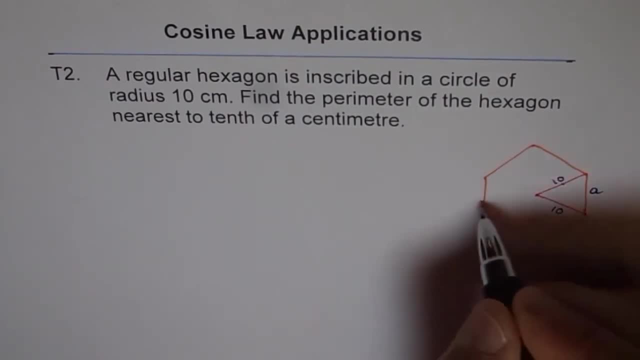 is 6 times A because all the sides are equal. correct, All the sides are equal and therefore we can find A right. Now couple of things here In a hexagon. what is going to be this angle? ok, Now, total angle is 360 degree, right, So we know the angle. let us say this is center. 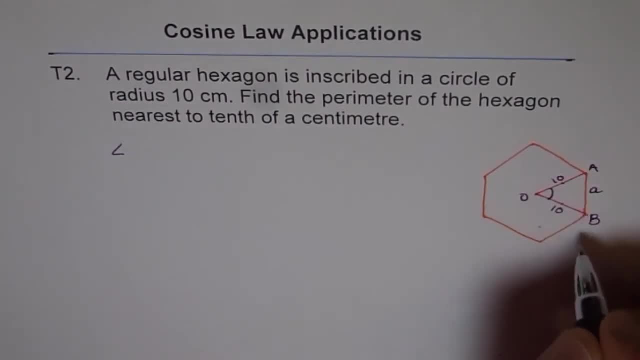 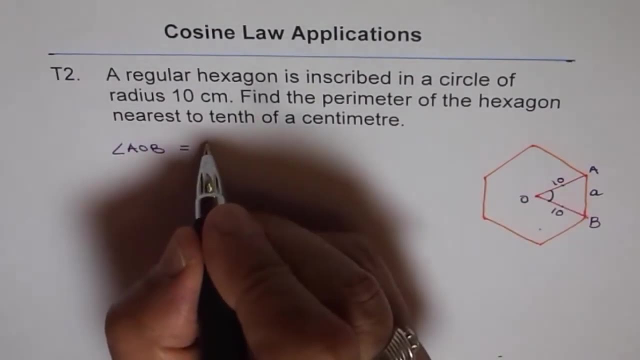 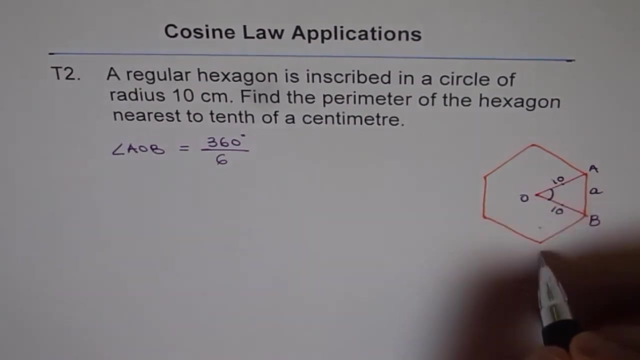 O and let us call this A and B as two point on this right. So the angle AOB should be equal to total divided by 360 degrees divided by 6.. Since these are 6 sides right, So we will have 6 triangles. That gives us an angle of 60 degrees. 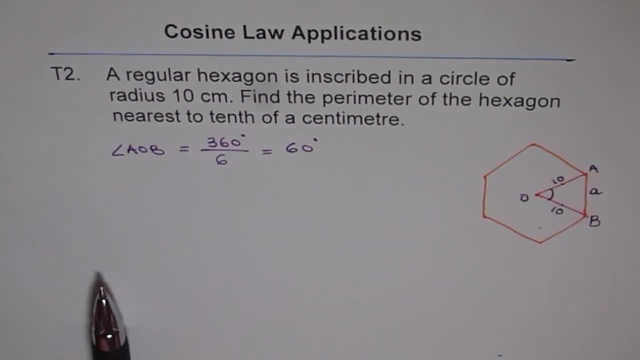 Ok, So we know this angle for us is 60 degrees, So we just found this to be 60 degrees. Now, if you know, 60 degrees is this angle and these are the two other sides given to you, You can always use cosine law and find what A is correct. That is so simple as this, Because 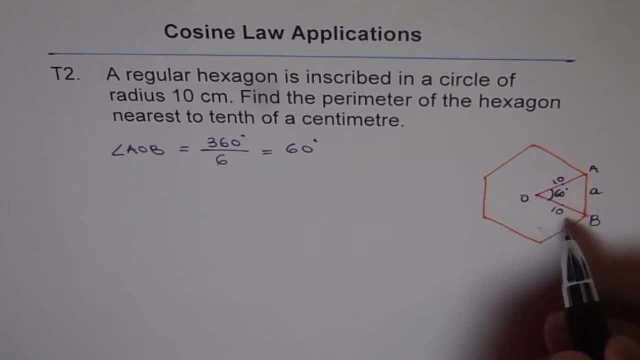 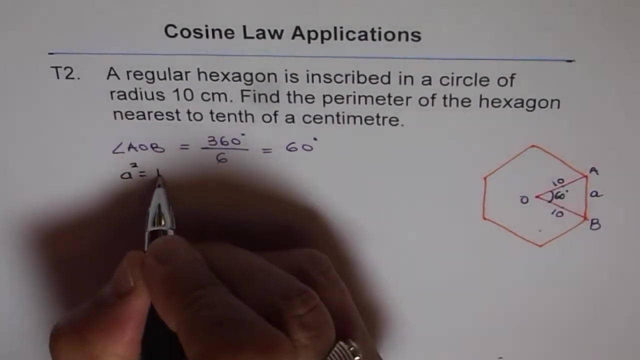 it is side angle side. So whenever it is side angle side, you cannot use side angle side. You can use مش건고. may not work for you In between 60 degrees. So we do not use side angle side guys. We are using side angle side. So we also can use cosine, because at the end 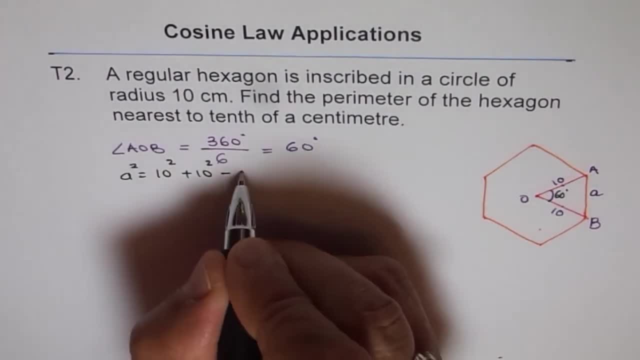 of our probability. we can use the dishwasher method, which is the graduating way, which is the positive constant plus sine dogs. So remember, we know that times 10 ten. Therefore, we can now find A equal to cosine law with sine, Yes, Okay. 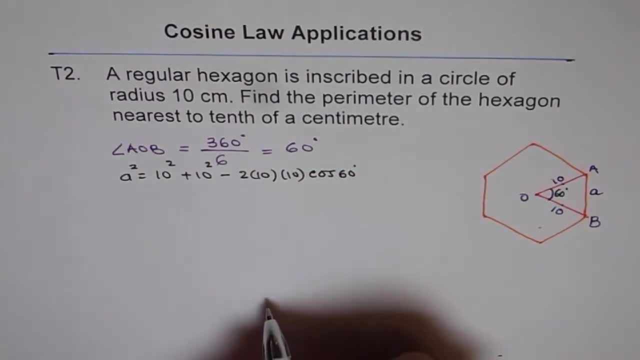 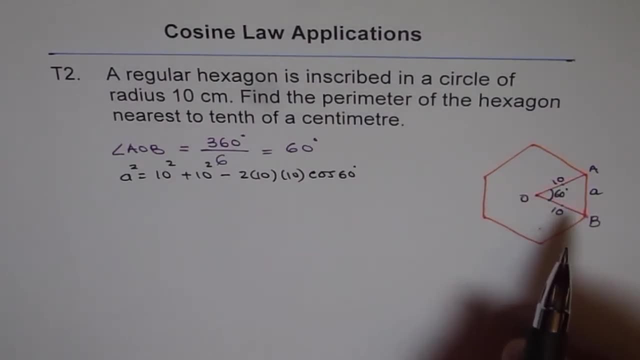 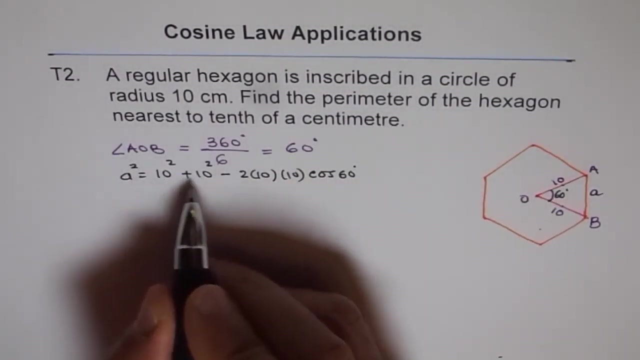 So the pentrukeu has two sides. utilize cosine law correct. So now we can find what is A equals to cos of 60 degrees. So that is your side square and you can always find the square root and figure it out right Now. cos of 60, you know, is half right and therefore we get this as 100 plus 100. 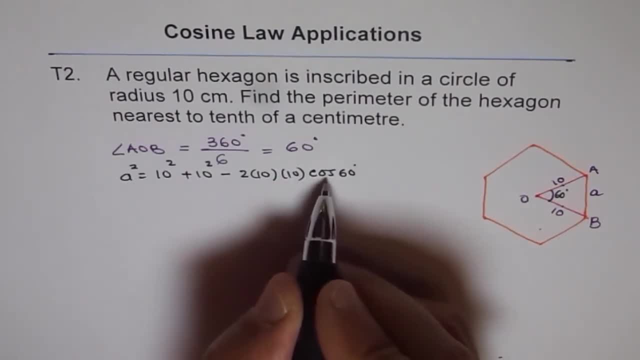 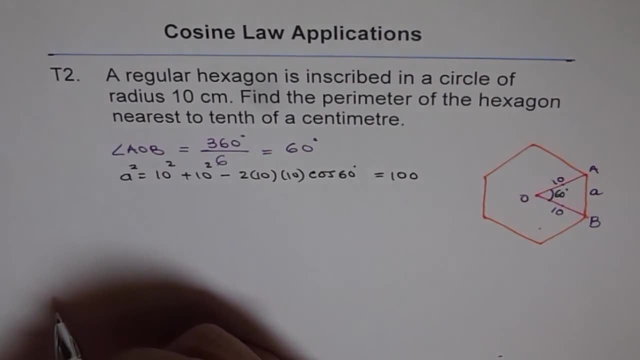 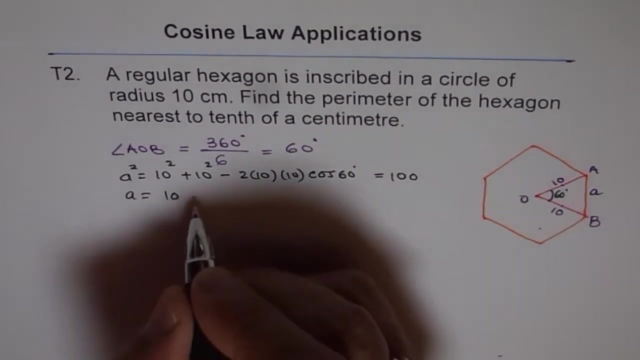 minus 200 times half is 100 and that gives you 100.. So these values are carefully taken so that there is not much calculation required. So a square root of 100, which is 10 correct, and therefore the perimeter is 10 times 6, correct, and we get perimeter. So we get perimeter is: 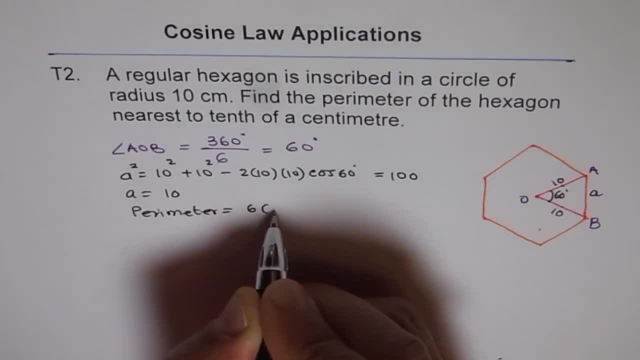 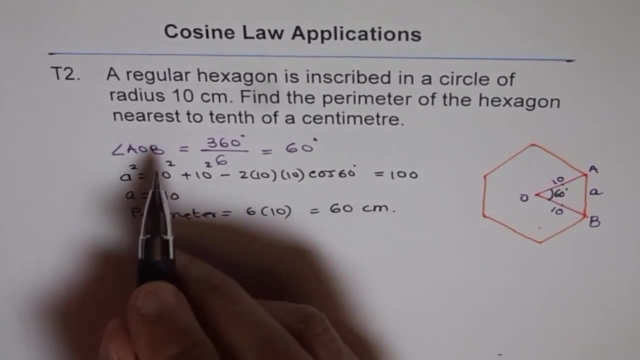 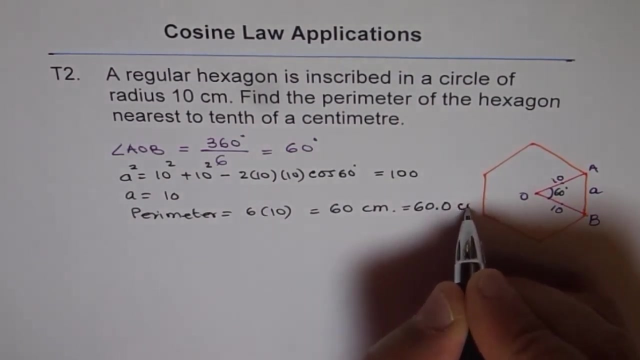 6 times 10.. There are 6 sides with a length, so that is 60 centimeter, correct, Nearest to the 10th of an centimeter '. Remember, we should write 60.0 cm as nearest to the 10th of a cm. 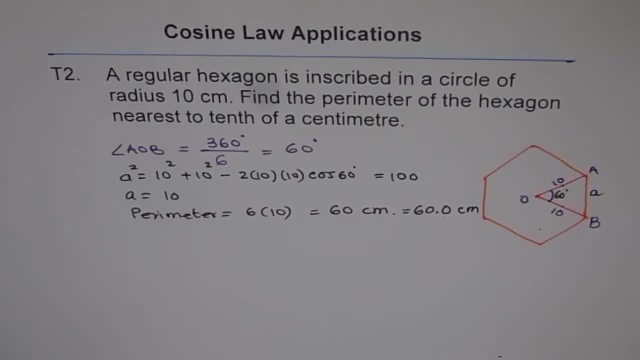 Well, this we did using cosine law, But we could have done the same question using sine law also. You know how? For sine law, we need these angles correct. Now, in this triangle, these two sides are equal. That means these angles will be equal. 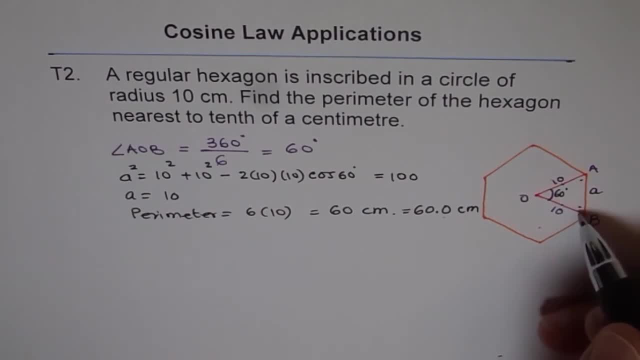 Now, sum of the angles is 180 degrees. Therefore, this angle should be how much? 180 minus 60 divided by 2.. That means 180 minus 60 is 120.. Divided by 2 is also 60.. 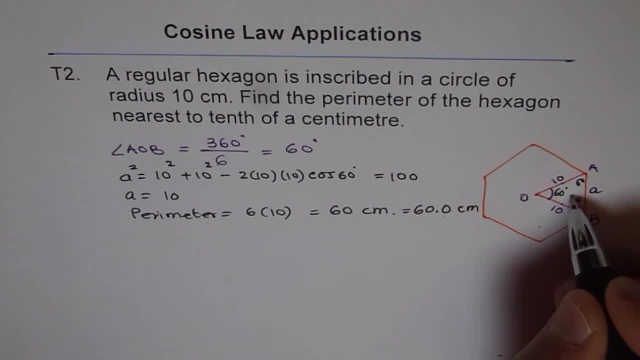 So we get these angles also at 60 degrees. Do you see that? So when these are 60 degrees, we know we can use sine law also, right. Or we can say: well, it's an equilateral triangle and side A is also 10.. 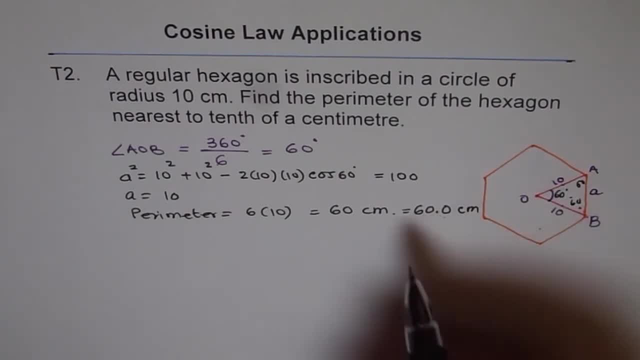 Correct, And therefore the perimeter is 60 cm. That is how we could do it, right? So we could do it in so many different ways in the same question, right? So that is how this problem can be done. 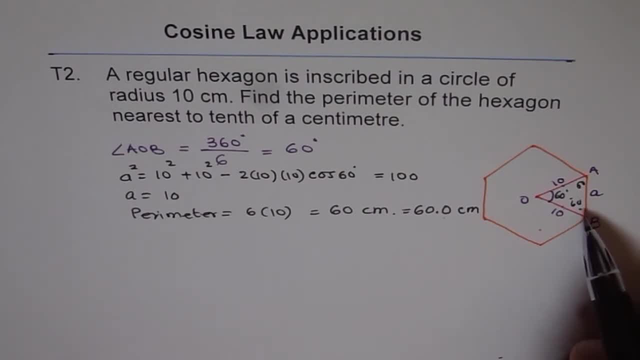 So you can actually do, even without sine law and cosine law, this problem, which looks very difficult, But once you sketch it and try to attempt it, it becomes very simple. I hope you enjoyed it. Thank you, Thank you.